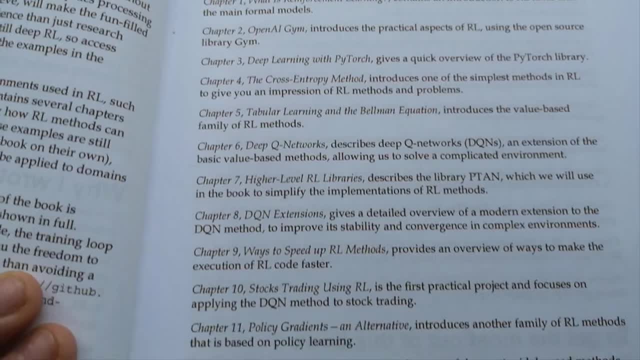 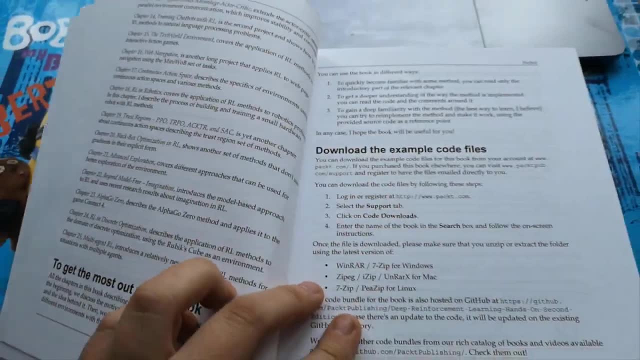 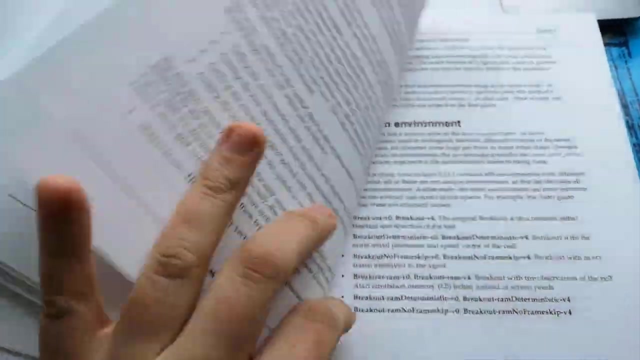 In the book. you can create a list of materials. You can use the book in different ways. To quickly become familiar with some method, you can read only the introductory part of the relevant chapter. Second, to get a deeper understanding of the way the method is implemented, you can read the code and the comments around it. 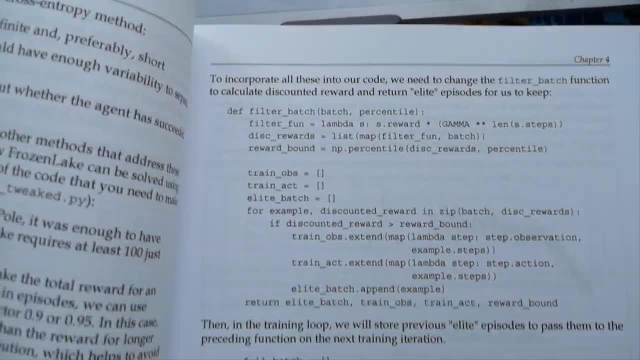 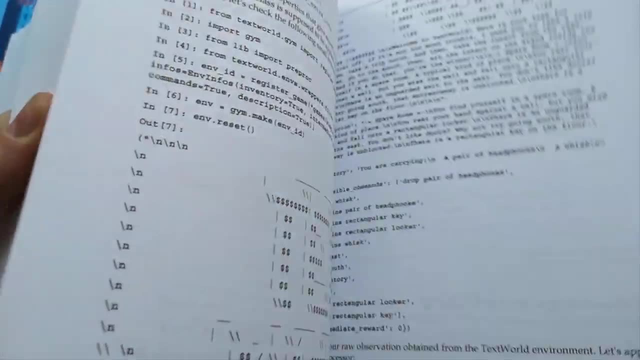 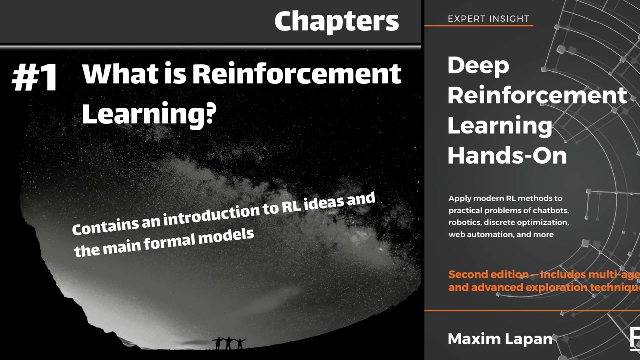 Last, to gain a deep familiarity with the method, you can try to reimplement the method and make it work Using the provided source codes as a reference point. the book has 25 chapters. chapter number one- what is reinforcement learning- contains an introduction to reinforcement learning ideas and the main formal models. 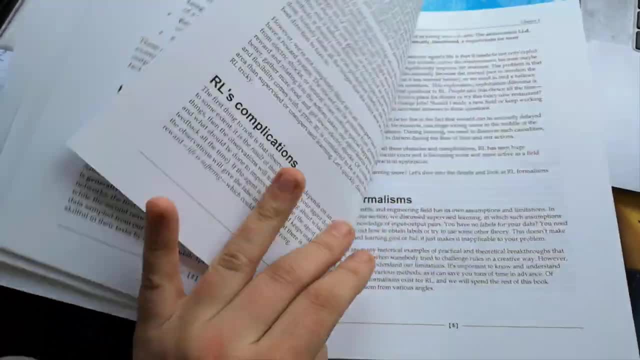 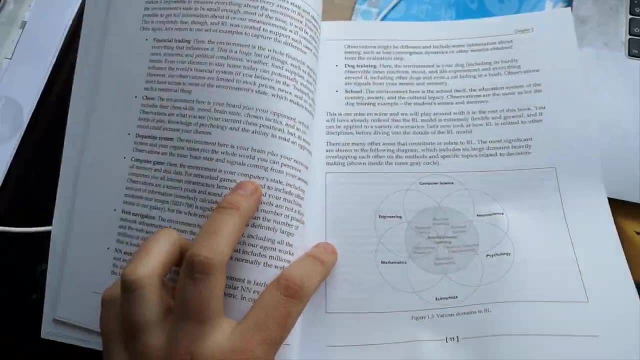 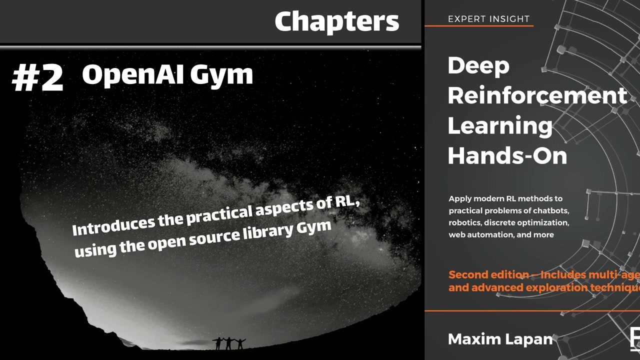 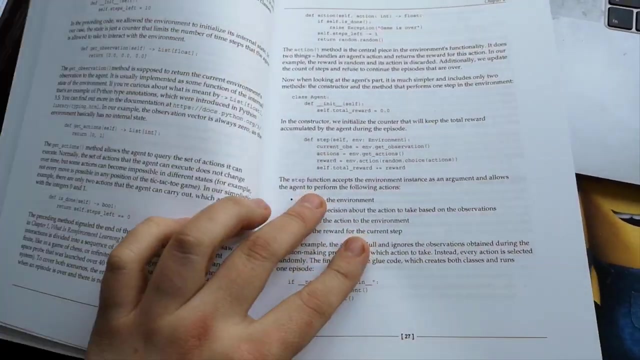 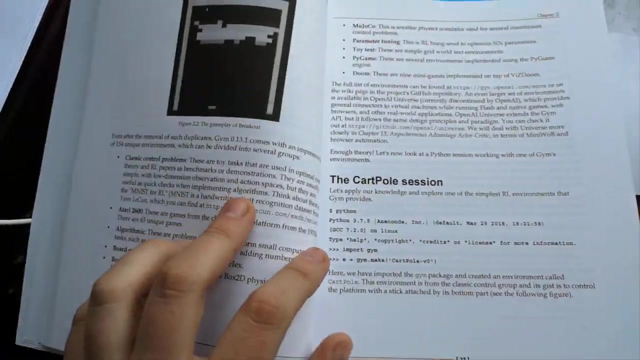 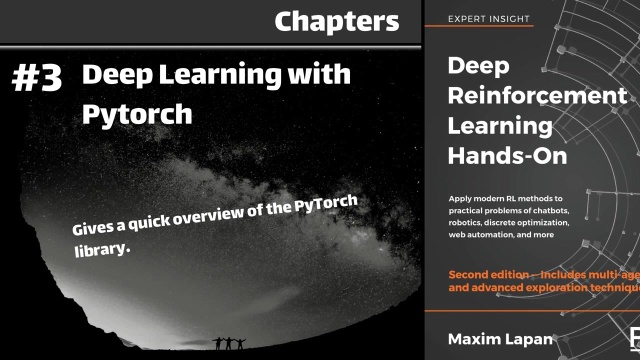 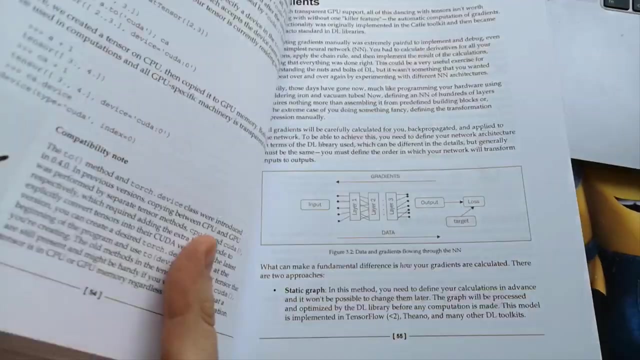 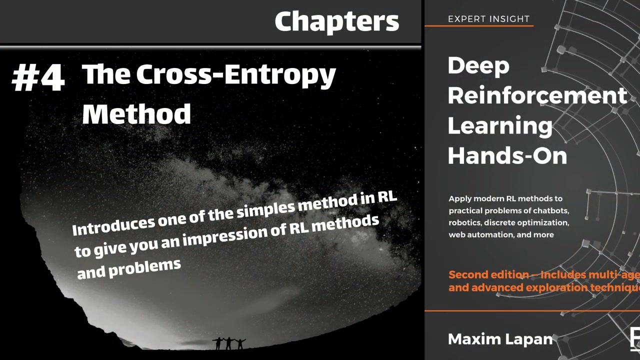 chapter number two: open ai gym introduced the practical aspect of reinforcement learning using the open source library gym you. chapter number three: deep learning with pytorch. give you a quick overview of the pytorch library. chapter number four: the cross entropy method introduces one of the simplest method of 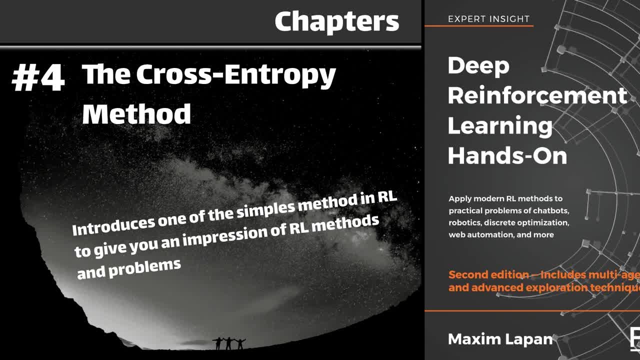 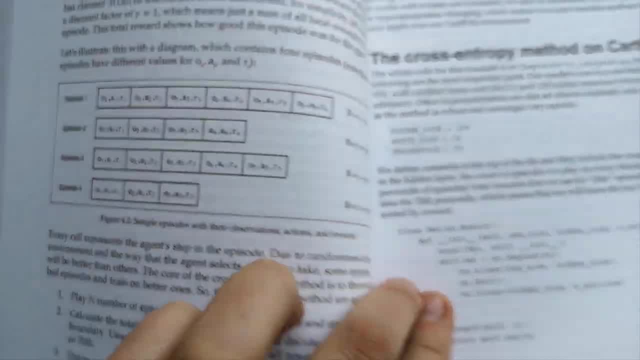 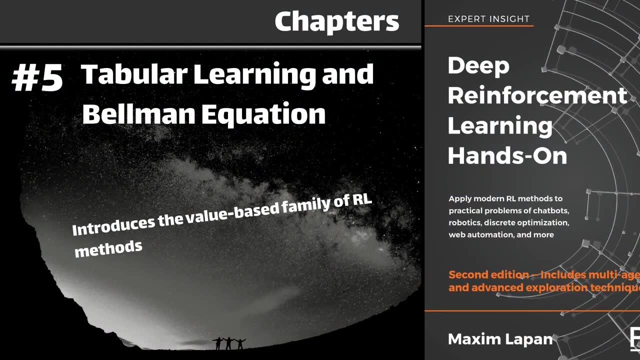 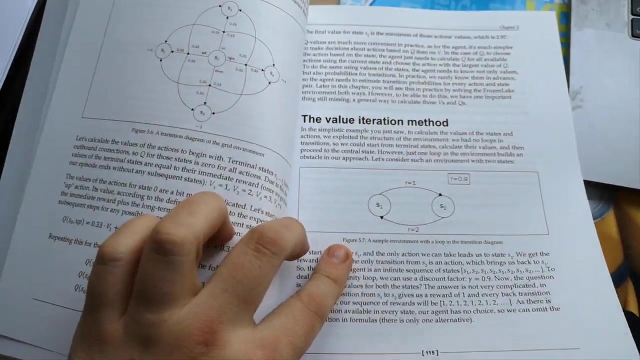 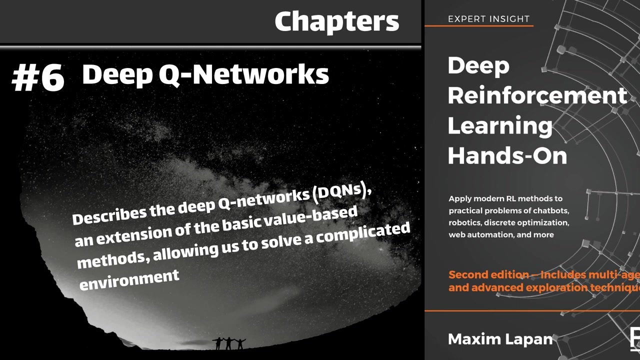 reinforcement learning. to give you an impression of reinforcement learning, of reinforcement method and problems, chapter number five, tabular learning and the bellman equation, introduces the value-based family of reinforcement method. chapter number six, deep q networks: describe deep q networks, dqns, an extension of the basic value-based methods. 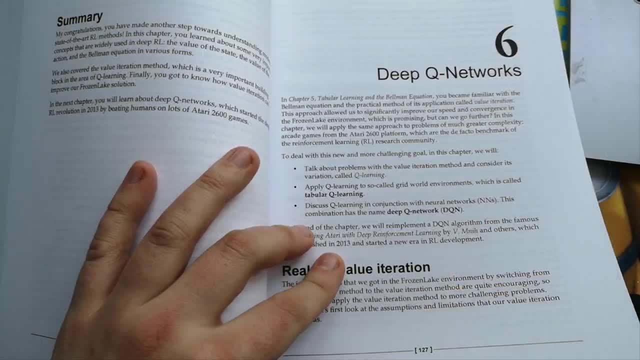 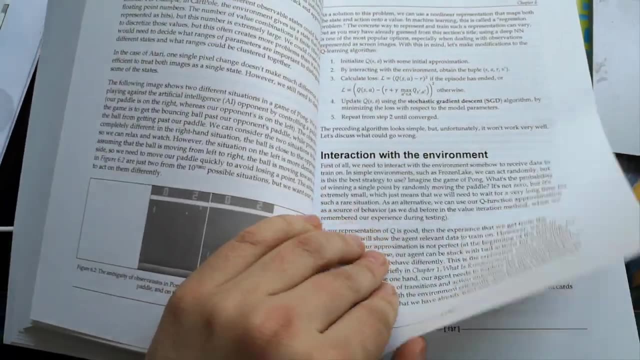 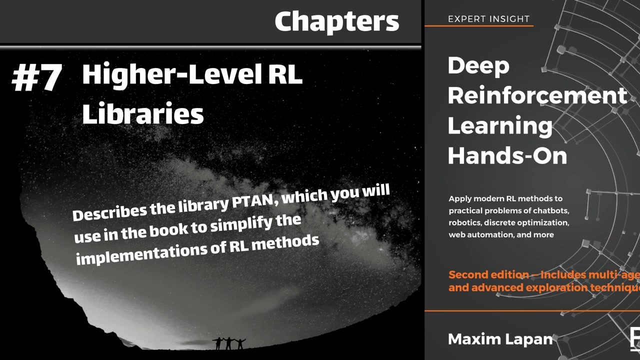 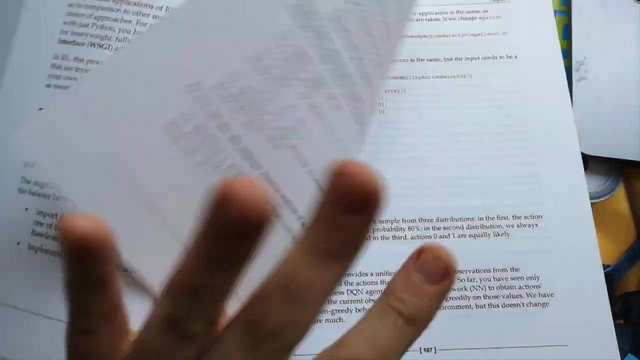 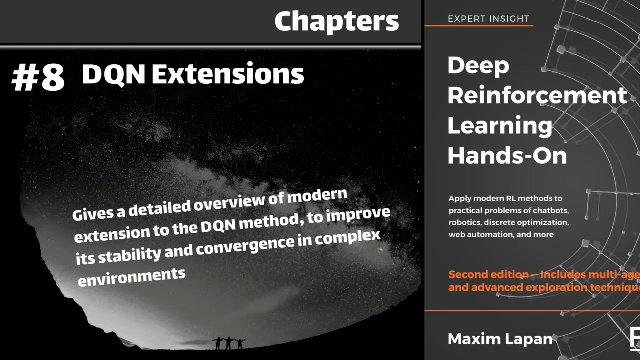 allowing us to solve a complicated environment. chapter number seven- higher level reinforcement learning libraries, describes the library p tan which we will use in the book to simplify the implementation of reinforcement learning methods. chapter number eight, tqn extensions, gives you a detailed overview of modern extensions to the 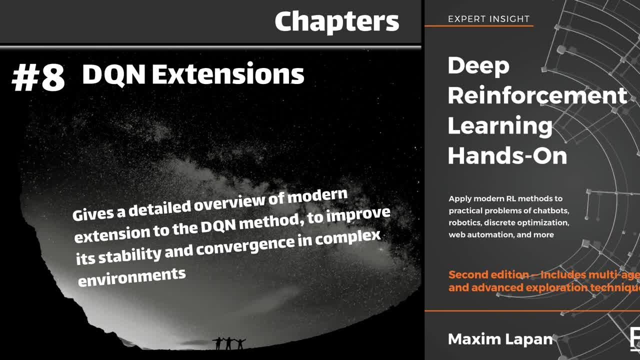 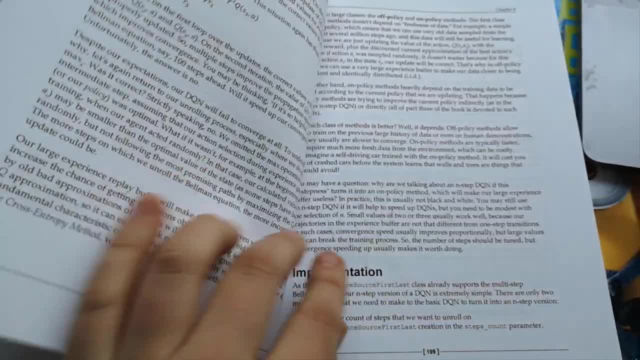 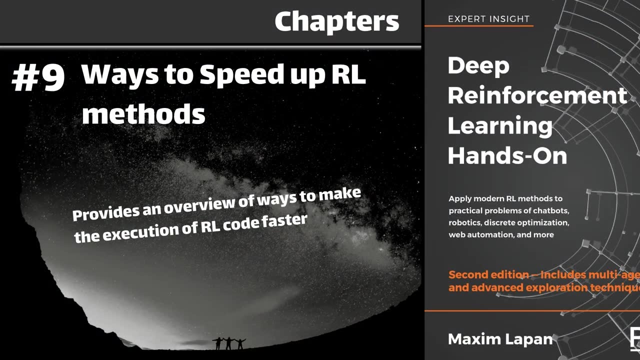 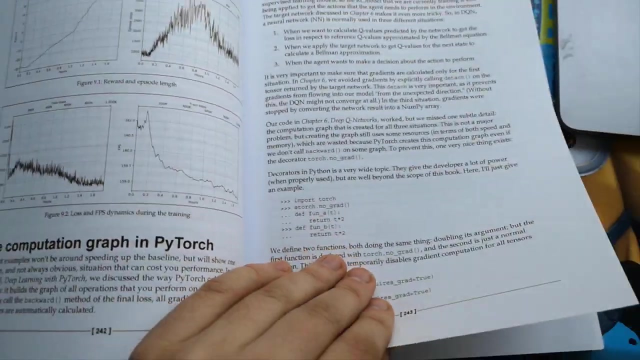 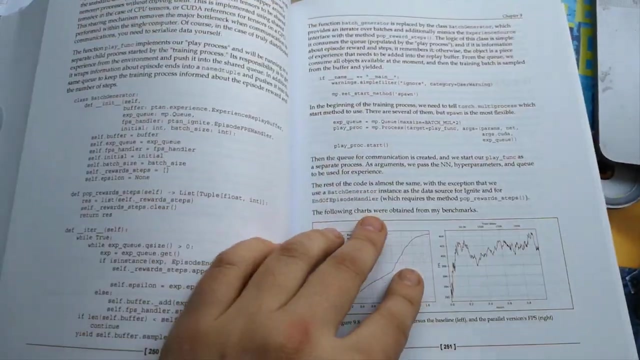 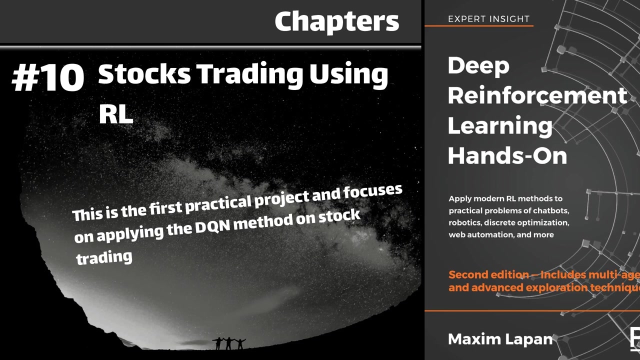 tqn method to improve its stability and convergence in complex environments. chapter number nine- ways to speed up reinforcement learning methods- provides an overview of ways to make the execution of reinforcement learning code faster. chapter number 10- stock trading using reinforcement learning- is the first practical project and focuses on applying the tqn method to stock trading. 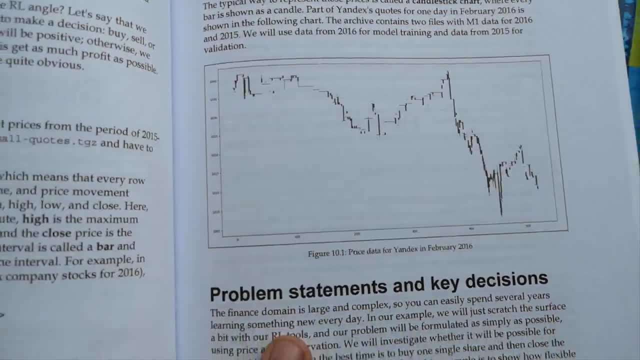 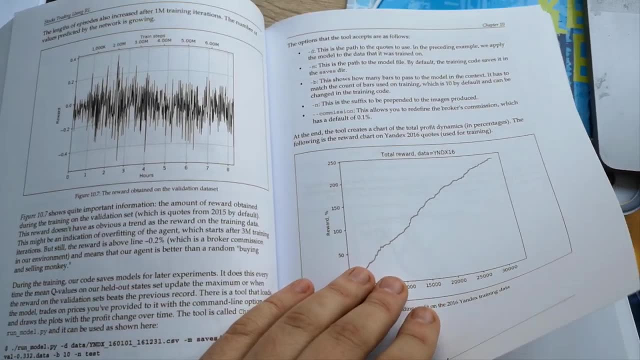 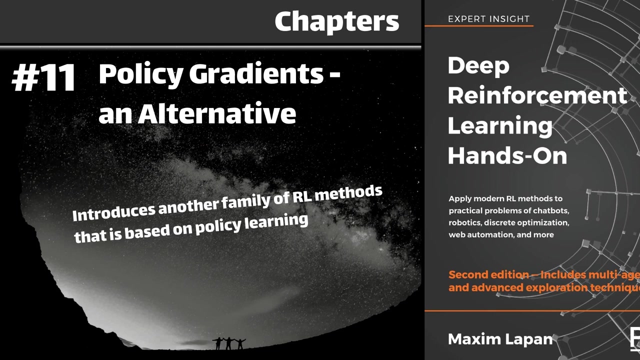 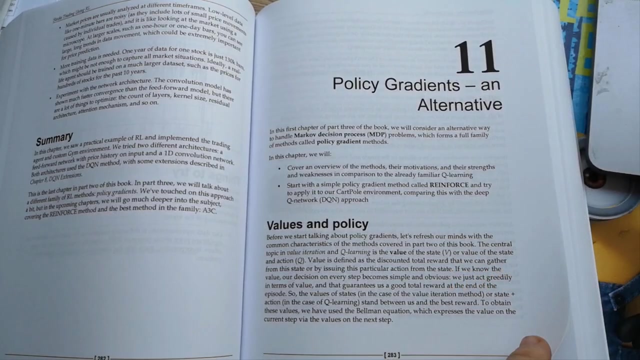 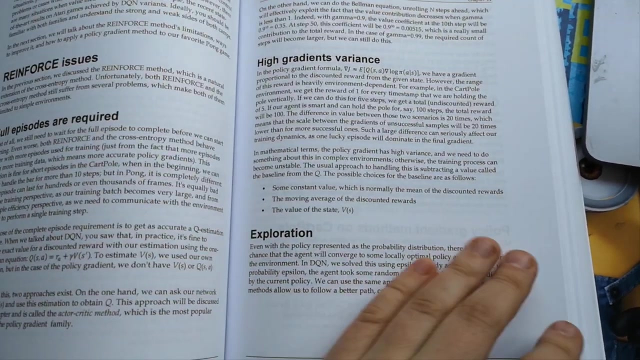 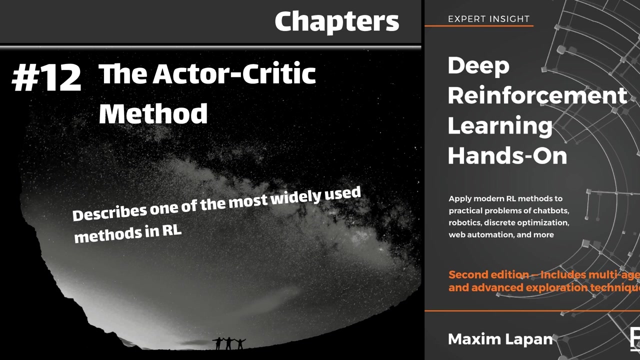 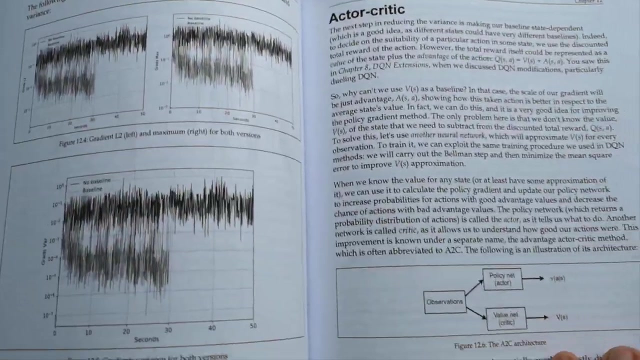 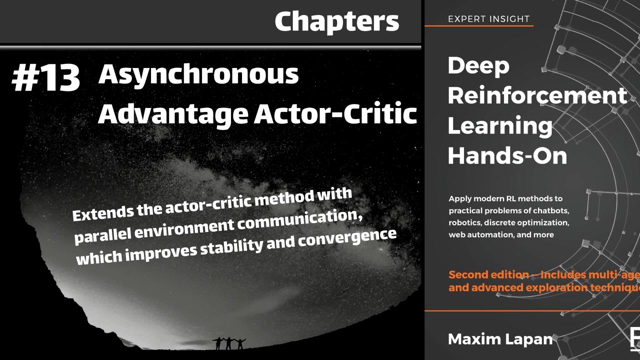 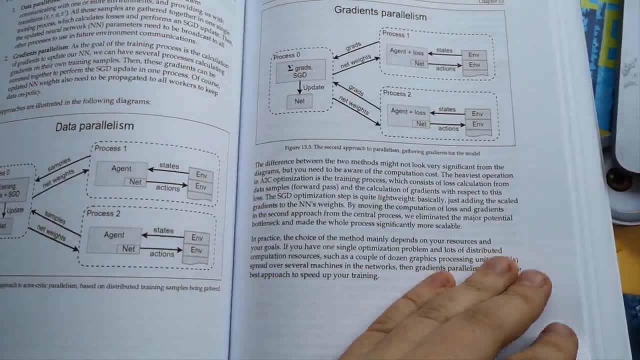 chapter number 13: asynchronous advantage actor critic extends the actor critic method with parallel environment communication, which improves stability and convergence. chapter number 13: asynchronous advantage actor critic extends the actor critic method with parallel environment communication, which improves stability and convergence. chapter number 13: asynchronous advantage actor critic extends the actor critic method with parallel environment communication, which improves stability and convergence. 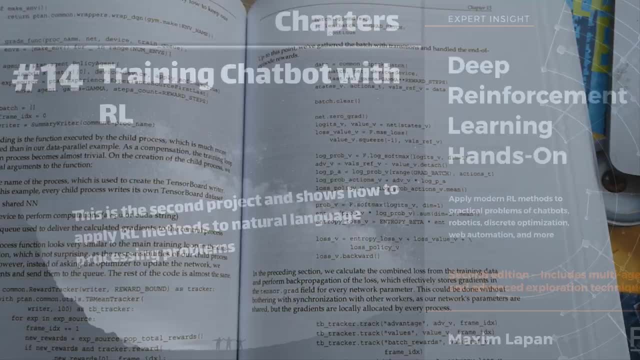 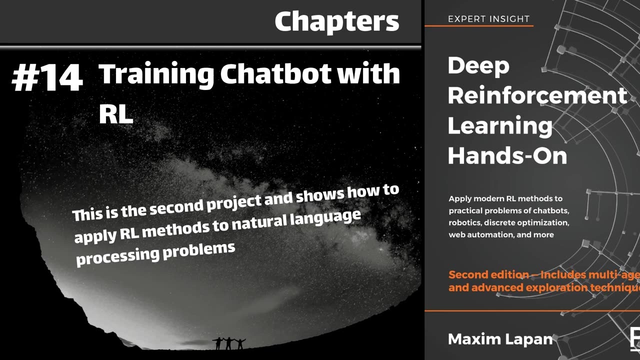 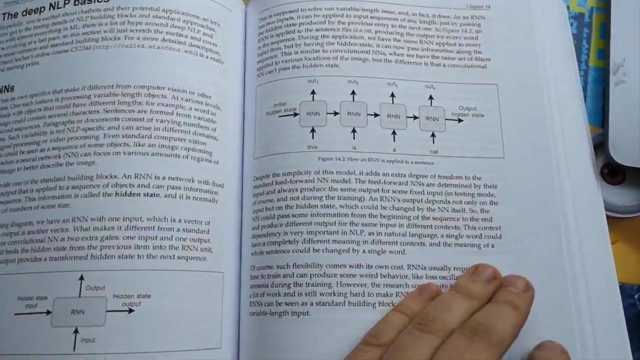 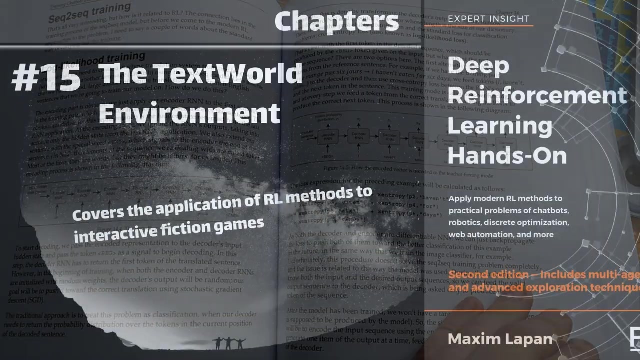 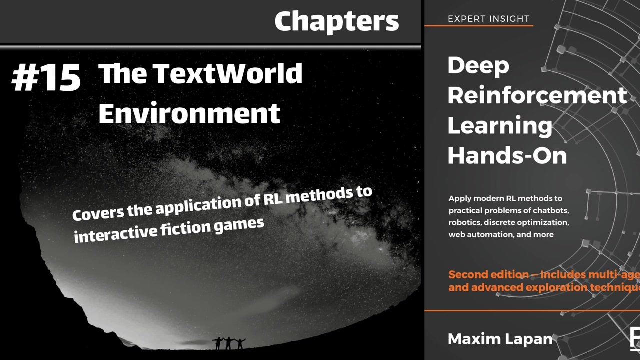 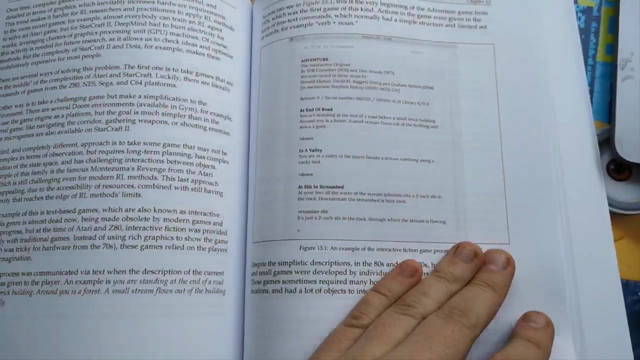 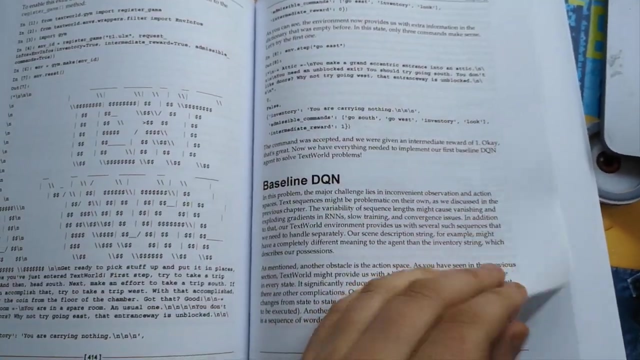 you, you, you. chapter number 14, training with reinforcement learning, is the second project and shows how to apply reinforcement learning methods to natural language processing problems. chapter 16- 19. Here's the application of reinforcement learning methods to interactive fiction games- Chapter number 16.. 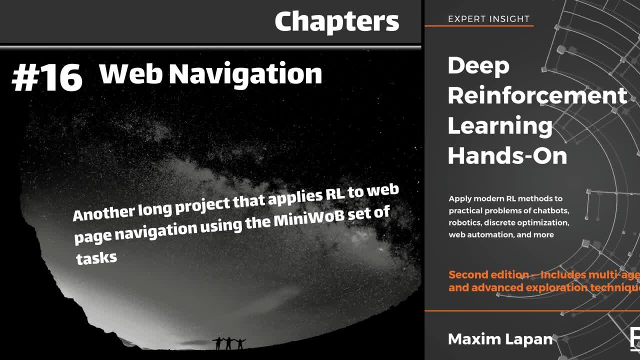 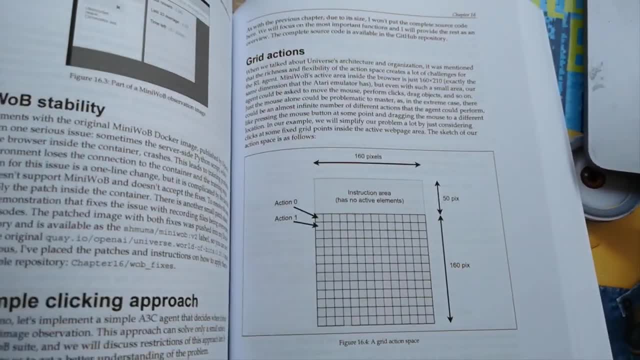 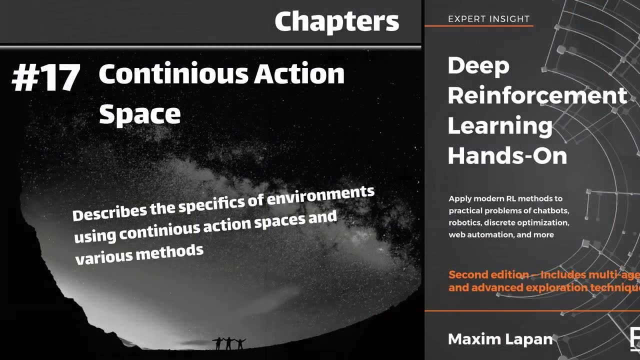 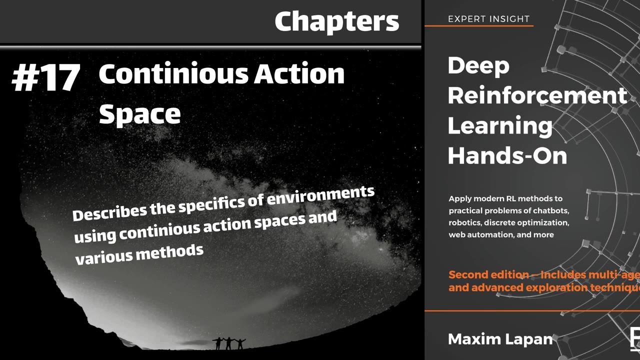 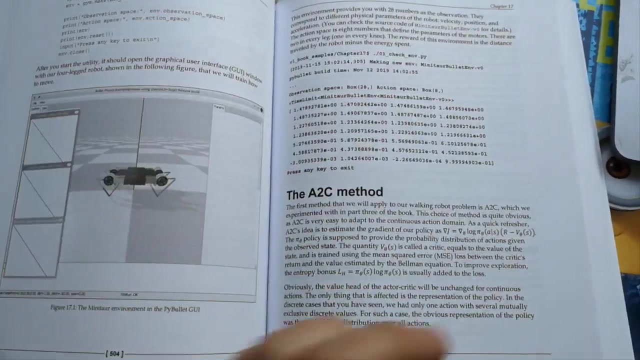 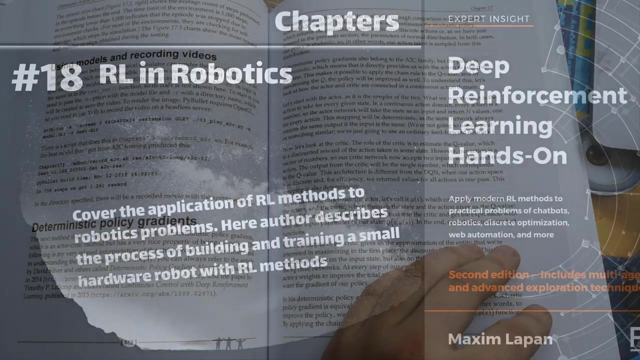 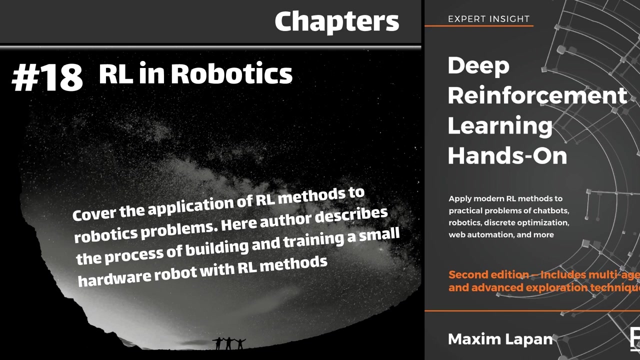 Web Navigation is another long project that applies reinforcement learning to web page navigation using the Mini-VoB set of tasks. Chapter number 17.. Continuous Action Space describes the specifics of environments using continuous action spaces and various methods. Chapter number 18. Reinforcement Learning in Robotic covers the application of reinforcement learning methods. 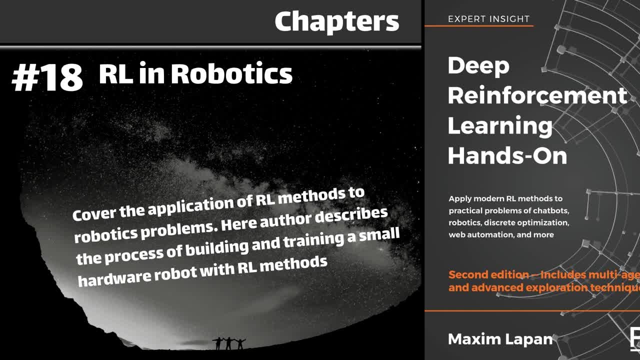 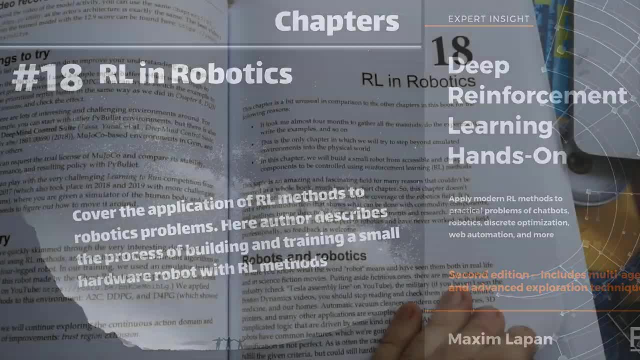 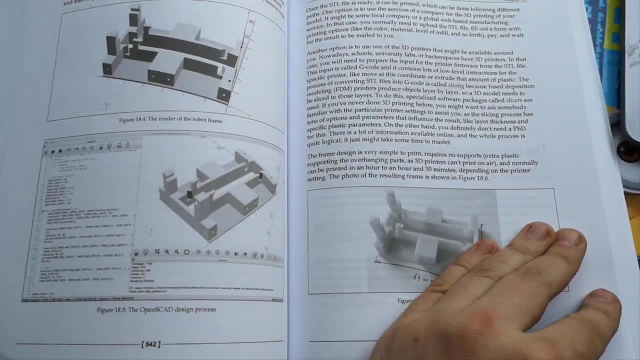 to robotic problems. In this chapter the author describes the process of building and training a small hardware robot with reinforcement learning methods- Chapter 18. Web Navigation is another long project that applies reinforcement learning to web page navigation using the Mini-VoB set of tasks. 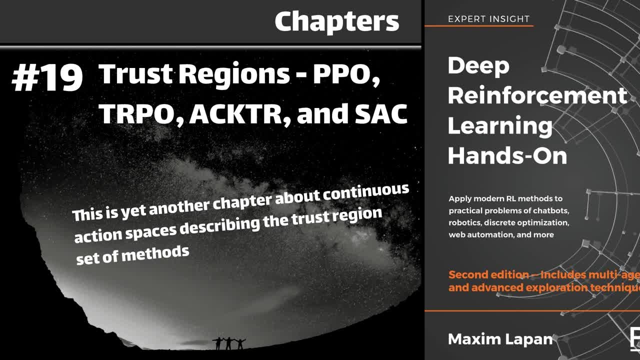 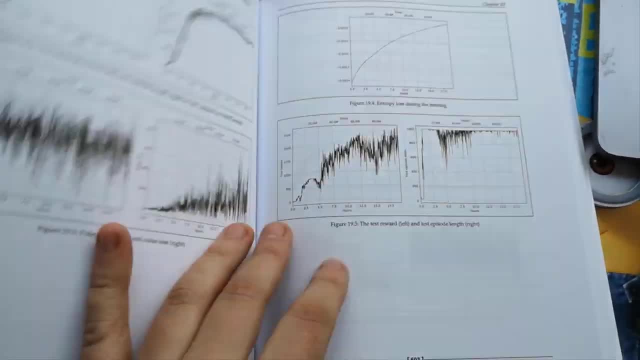 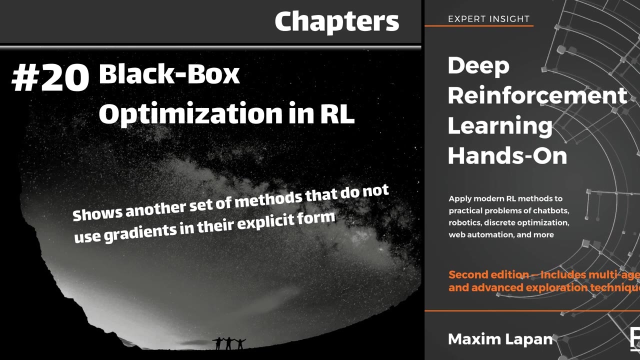 Chapter number 19. Trust Regions- PPO, TRPO, ACKETR and CAC is yet another chapter about continuous action spaces describing the Trust Region set of methods, Chapter 19. Black Box Optimization in Reinforcement Learning shows another set of methods that don't. 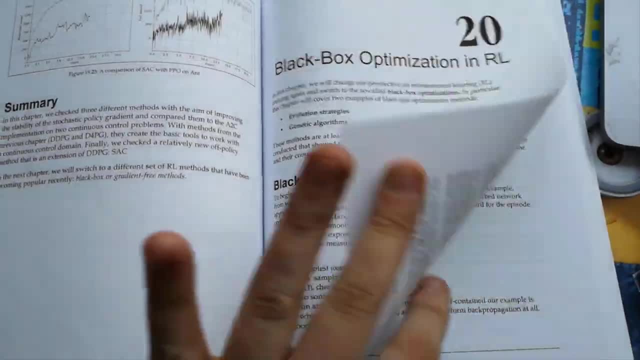 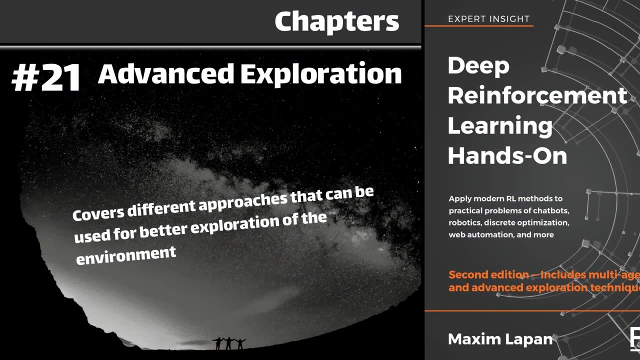 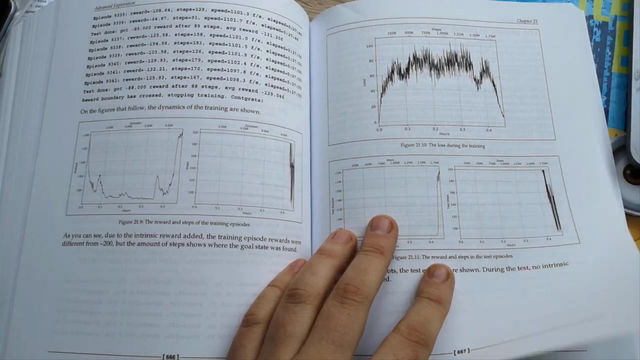 use gradients in their explicit form. Chapter 21. Advanced Exploration covers different approaches that can be used for better exploration of the environment. Chapter 20. Black Box Optimization in Reinforcement Learning shows another set of methods that don't use gradients in their specific form. 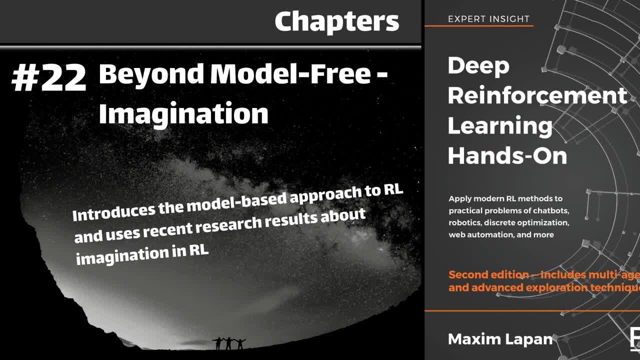 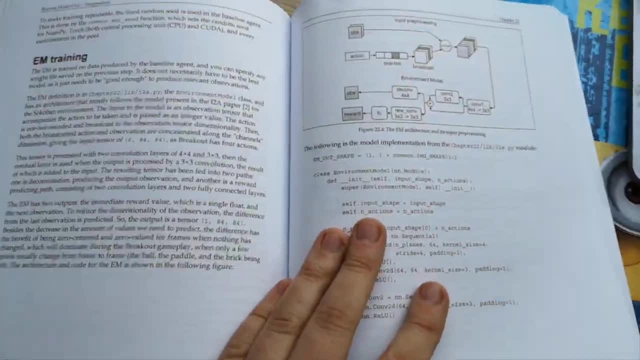 Chapter 21. Beyond Model 3. Beyond Model 3 Introduces the model-based approach of reinforcement learning and uses recent research results about imagination in reinforcement learning. Chapter 22. comment yourself, Learn more. Thank you, Have a nice day. 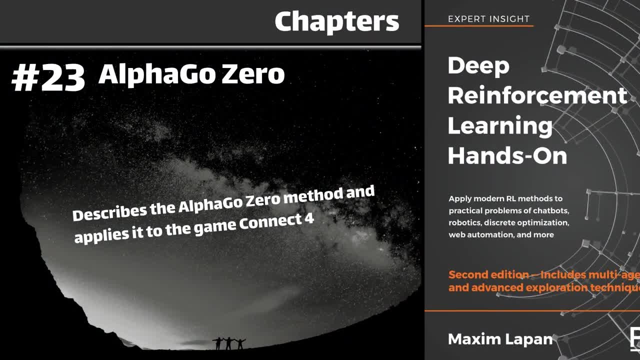 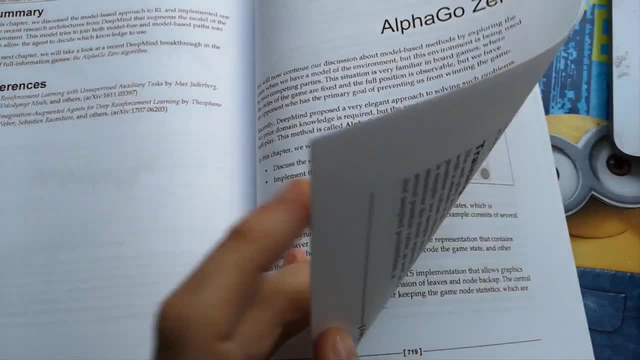 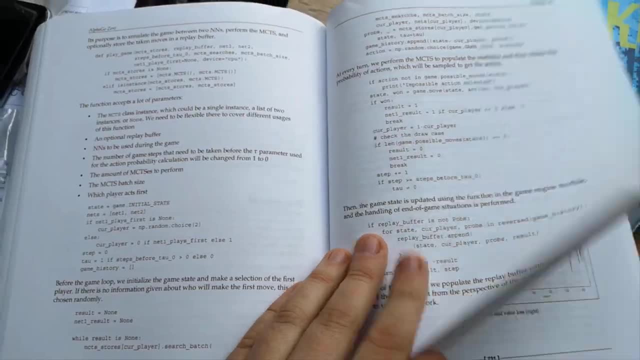 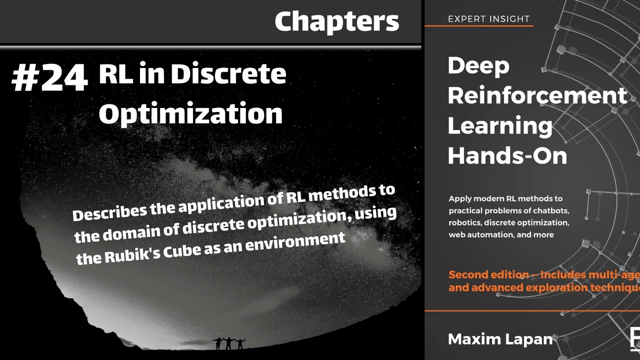 Chapter number 23.. AlphaGo Zero Describes the AlphaGo Zero method and applies it to the game Connect4.. Chapter number 24.. Reinforcement Learning in Discrete Optimization Describes the application of reinforcement learning methods to the domain of discrete optimization. 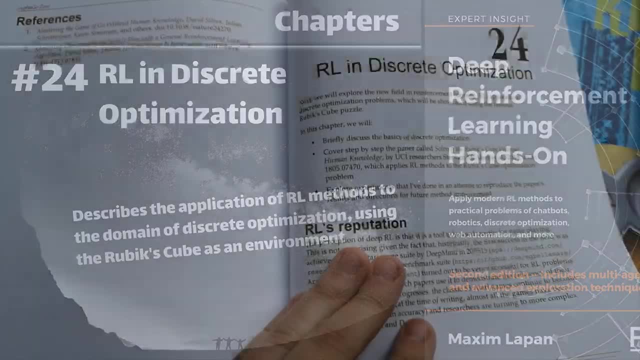 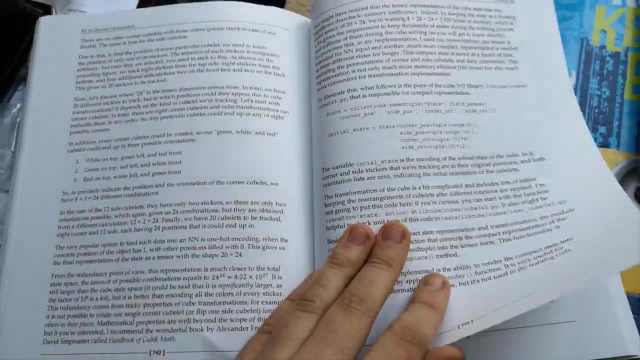 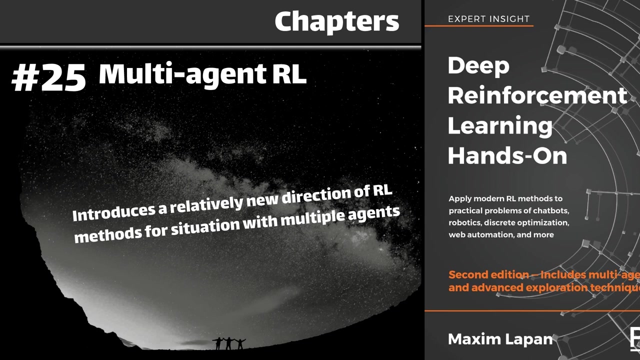 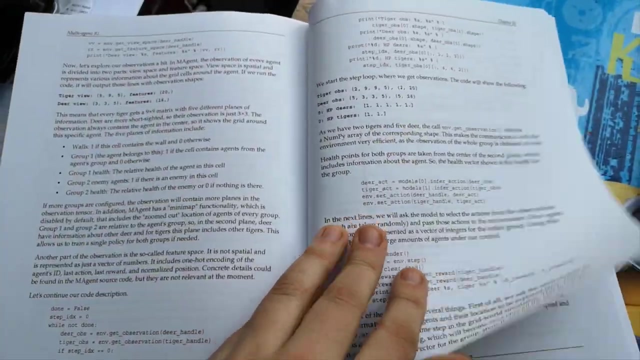 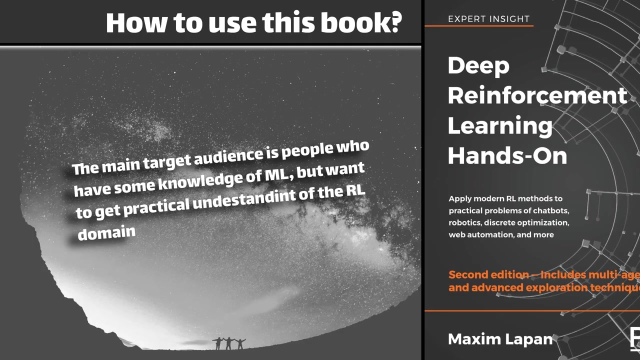 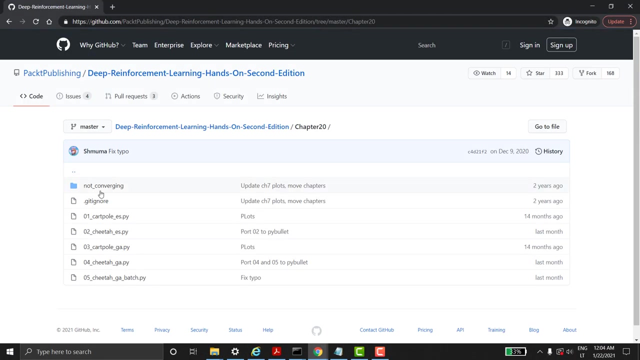 Using the Rubik's Cube as an environment. And last one, Chapter number 25.. Multi-agent reinforcement learning introduces a relatively new direction of reinforcement learning methods for situations with multiple agents. You can download the code for the book from the internet and all the codes are hosted in GitHub and there you can use this code for your project and use the same step as is provided in this book. 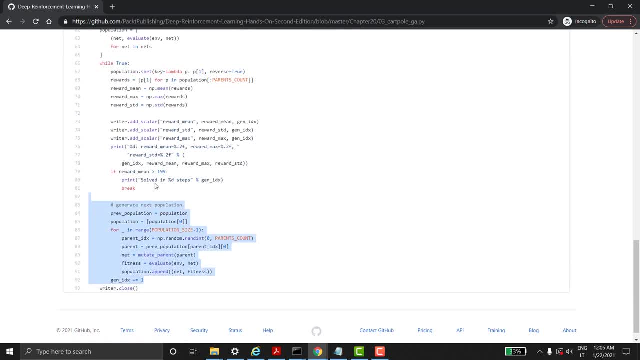 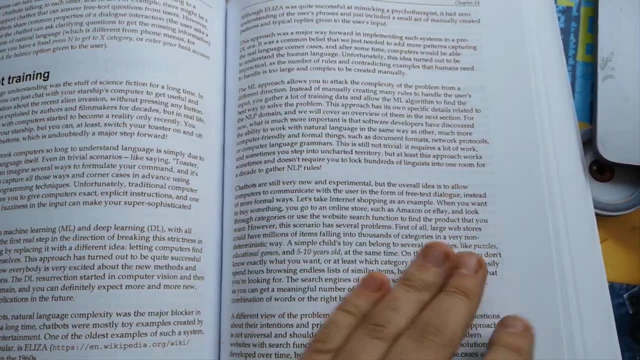 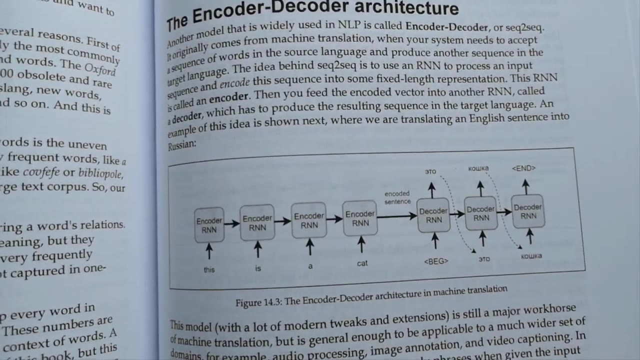 This book is an updated and expanded version of the best-selling guide to very latest reinforcement learning tools and techniques. It provides you with a lot of information about reinforcement learning methods and how to use them. It provides you with an introduction to the fundamentals of reinforcement learning, along with the hands-on ability to code intelligent learning agent to perform a range of practical tasks.